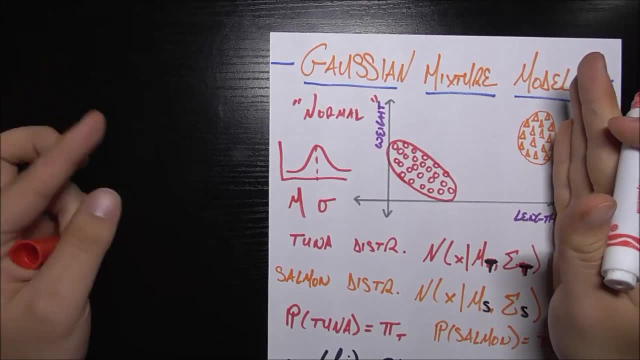 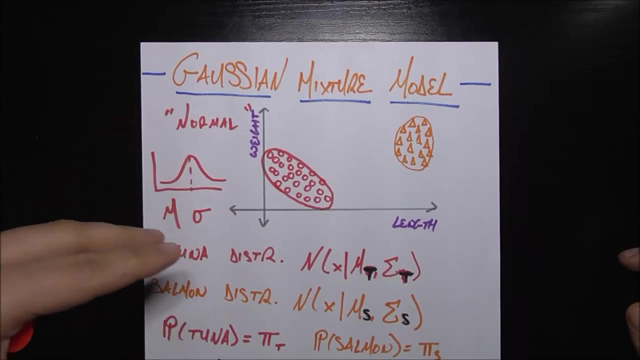 distribution. So a high sigma would mean that it's very spread out. a low sigma would mean that it's pretty compact, right? So in the same way, when we have higher dimensions, probably you would want to study the multivariate normal distribution before going through this video. but in higher dimensions, 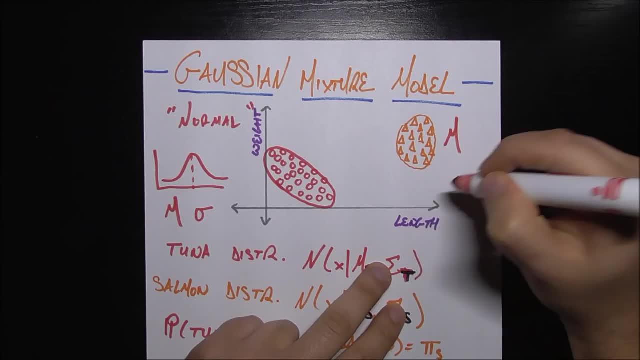 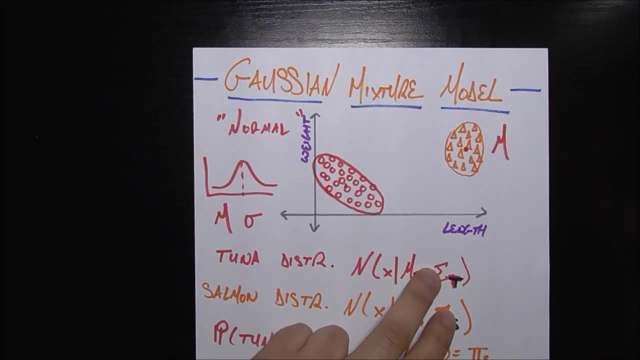 it's the same form. we have a mu vector now, so here it's a two-dimensional vector. The mu for salmon is probably something around there the middle of that, the mu for tuna is probably something around there the middle of that. and we have, instead of sigma, which is our standard standard deviation. 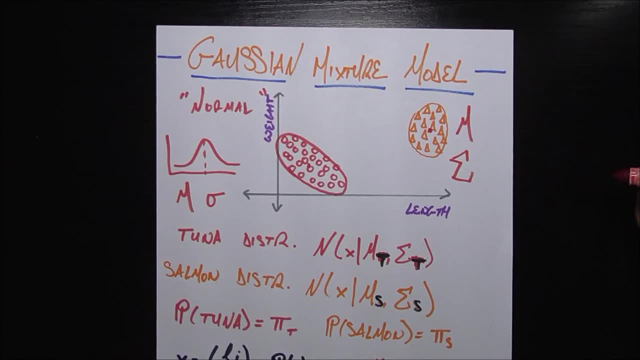 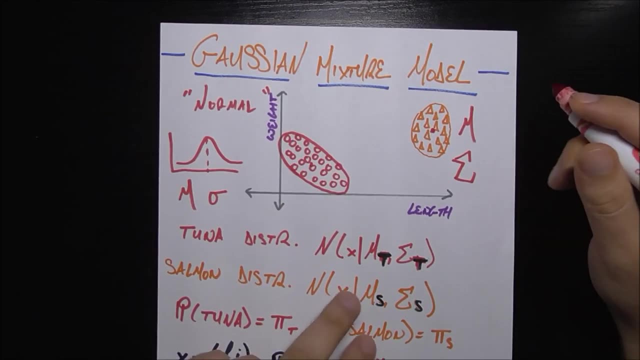 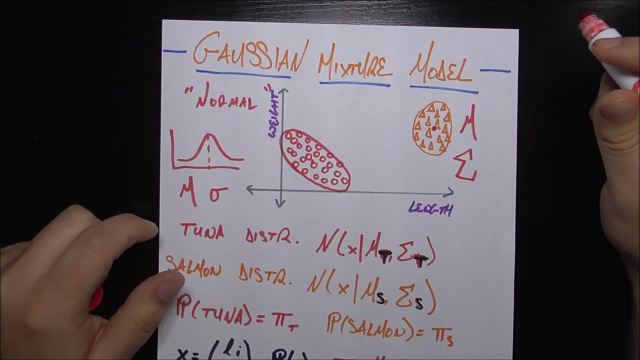 we have a covariance matrix sigma. okay, So this is capital sigma and this is a 2x2 matrix, because we're in two dimensions and it basically just tells us what's the shape of that oval. So is it more circular, Is it more of an oval, Is it tilted, Is it not tilted? That's what the entries of sigma. 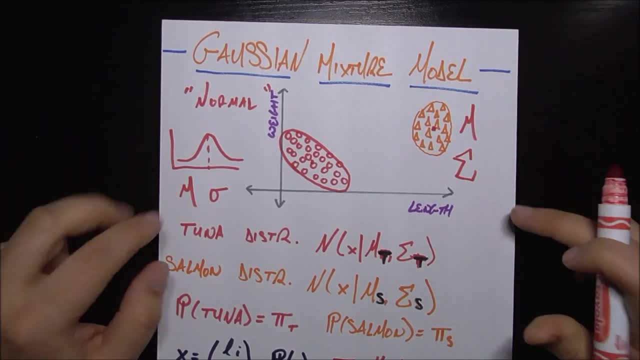 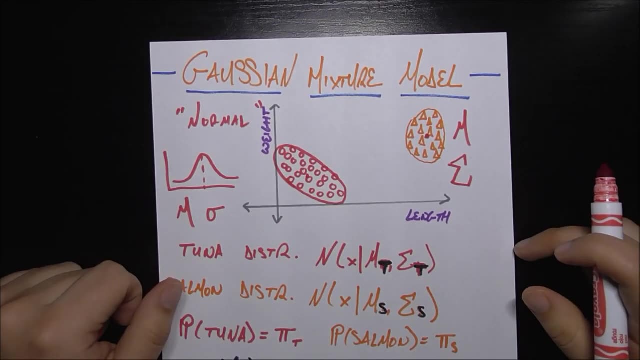 basically tell us at a very high level. okay, So again, the Gaussian mixture model assumes that our classes, in this case our two classes, are Simon and Tuna. our classes are distributed in a normal distribution in however many dimensions we have data for Here we have two dimensions. 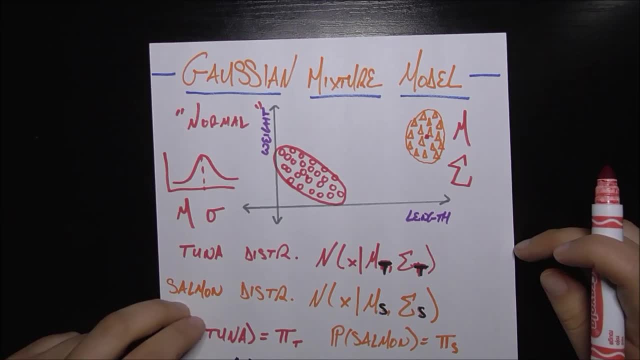 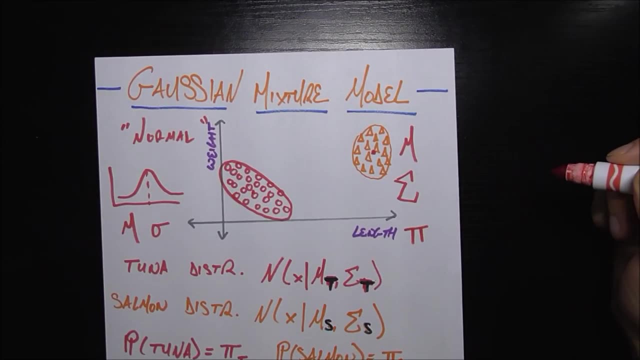 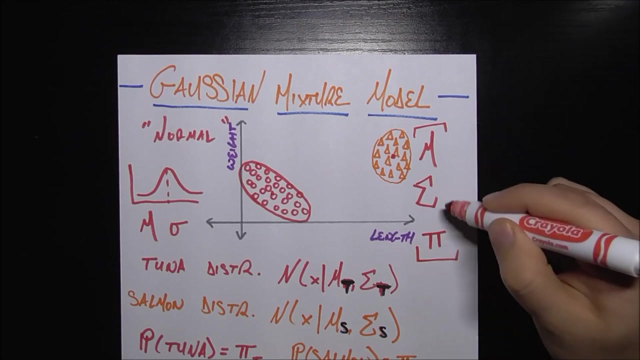 of data. So the goal is trying to figure out the best parameters. so the best mu, sigma, and there's another parameter called pi, and this one simply just tells us what's the probability of being in either class- Simon or Tuna. So we have these three sets of parameters, the pi's- 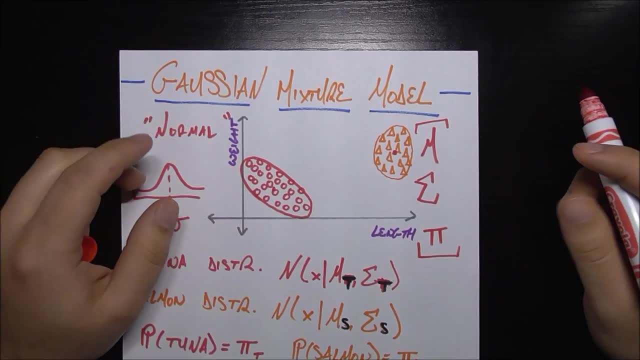 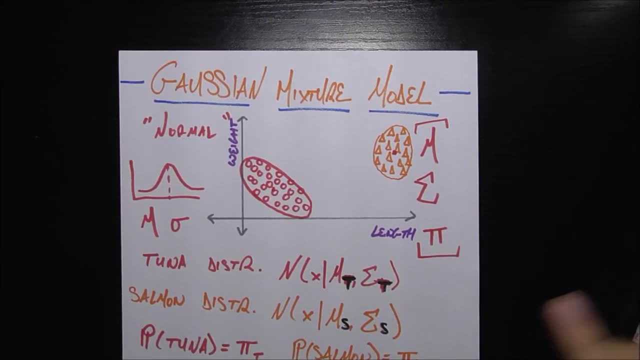 the sigma's and the mu's. The Gaussian mixture model tries to figure out the optimal values of these parameters to best fit our existing data, so that if a new data point comes in, I'm going to say this is a new data point. Obviously, we think it goes to the salmon because it's really within. 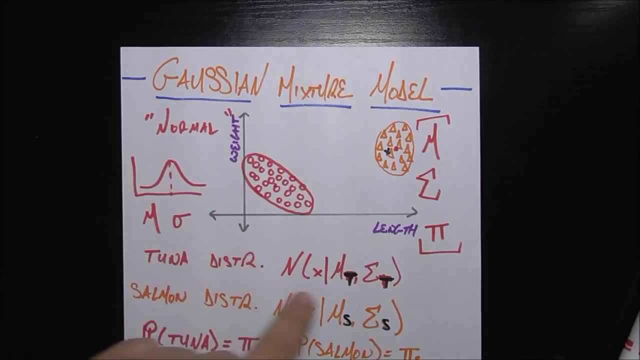 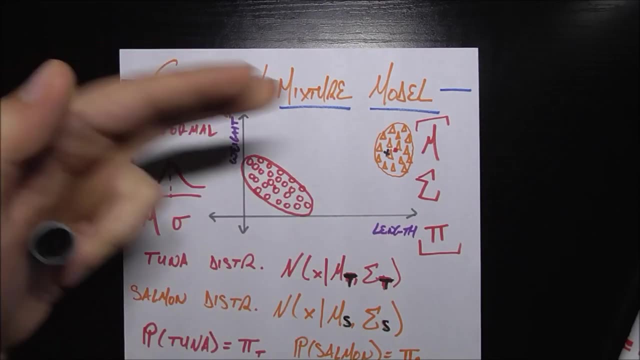 that distribution, but based on the optimal parameter. we're going to say it's a new data point. So if we look at the parameters we find with our existing data, we should be able to mathematically determine that that new point, with its length and its weight, should be in the salmon. 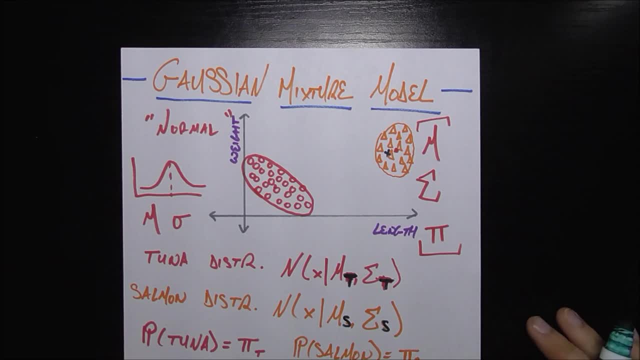 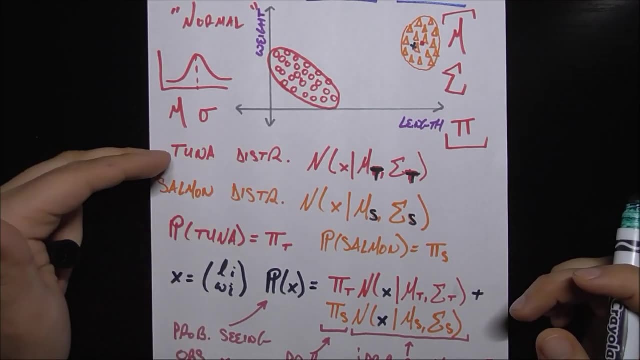 distribution. okay, So that's at a high level how the Gaussian mixture model works. Let's go into some of the more math of it. So again to break it down, it assumes that there's some Tuna distribution which is distributed normally with mu t. mu sub t is the mean for Tuna, which again 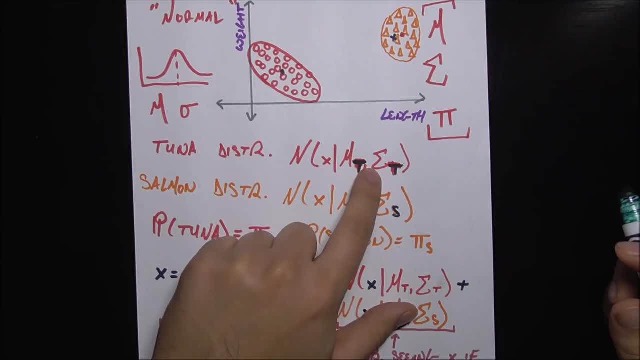 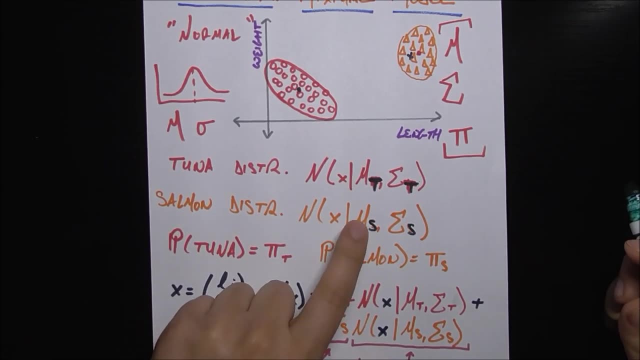 is probably something around there- and sigma sub t, which is the covariance matrix for the Tuna normal distribution. We also assume that there's a salmon distribution with some other mean mu sub s and some other covariance matrix. sigma sub s, This x, if you're wondering, is simply 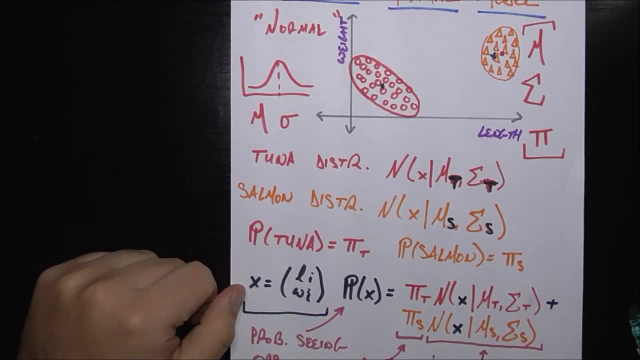 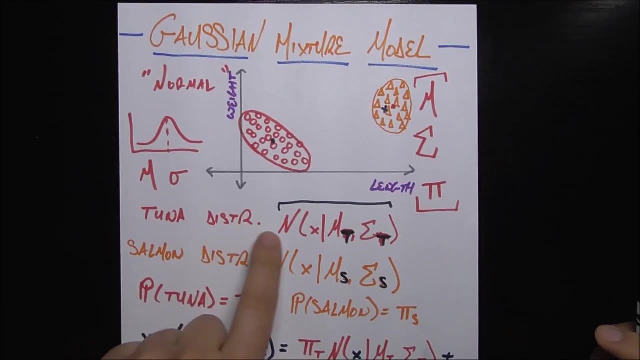 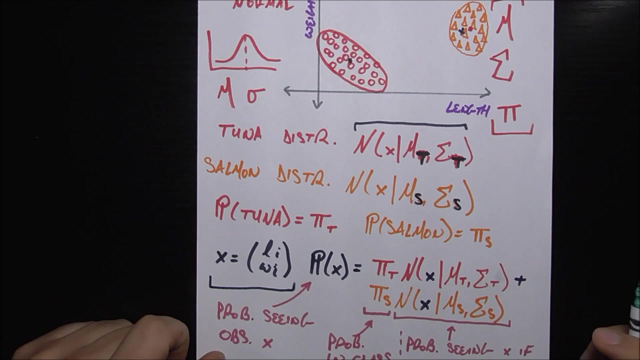 just the vector which tells us the length and the weight of any fish. So this line basically here means that if I know that something is a Tuna, then I know that it's distributed according to mu sub t and sigma sub t, And again there's also these pi parameters. 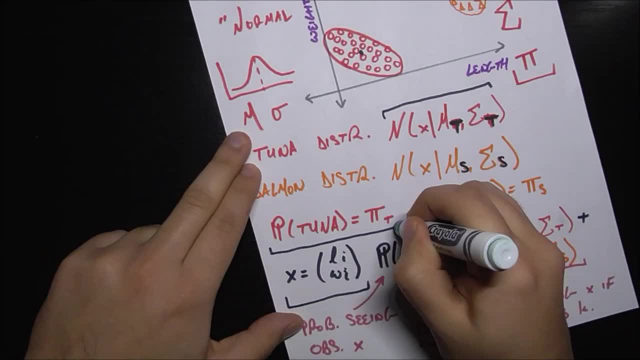 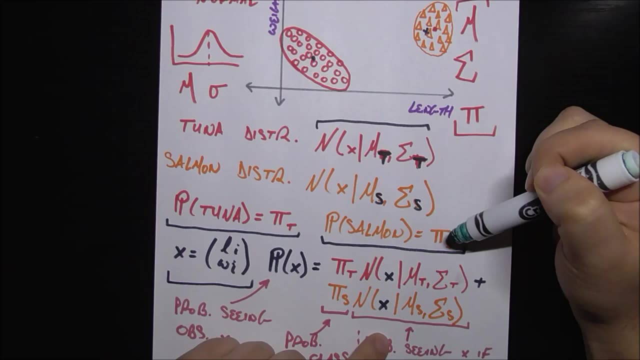 which basically tell us what's the probability that something is a Tuna? that would be pi sub t, and probability that something is a salmon would be pi sub s. So these parameters together, mu, sigma and pi, completely describe our entire situation here. Now how do we figure? 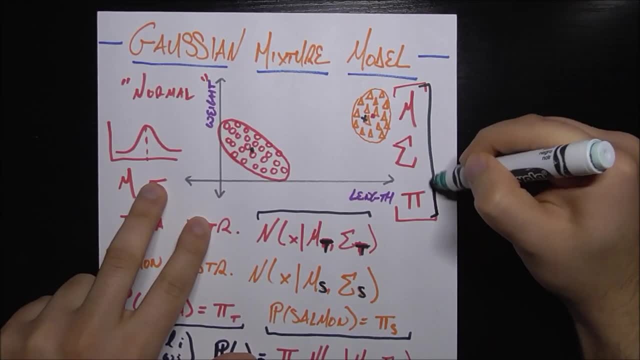 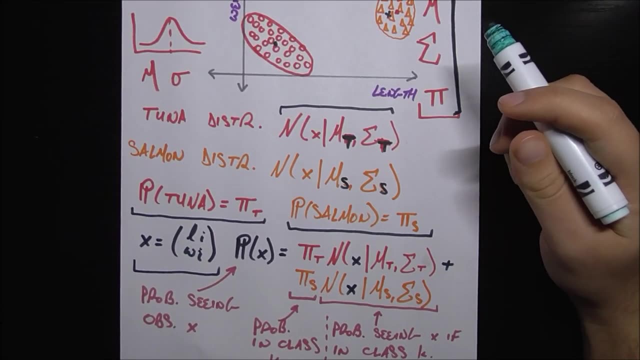 out these best parameters. right, That's our goal. Once we figure out these parameters, it'll be pretty easy to figure out whether a mystery thing is a salmon or a tuna. Well, we want to maximize a certain quantity, and that quantity is right here, this probability of x. So 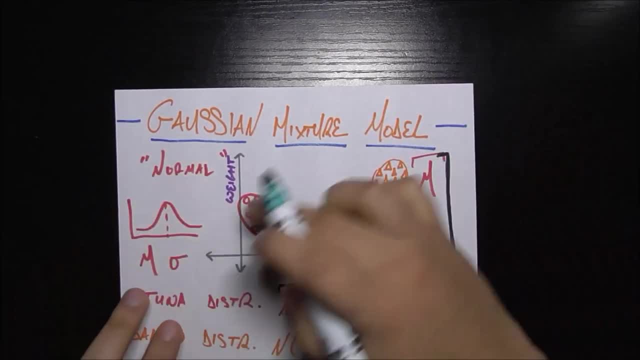 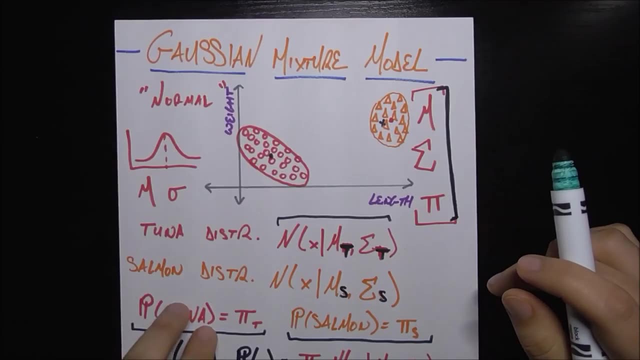 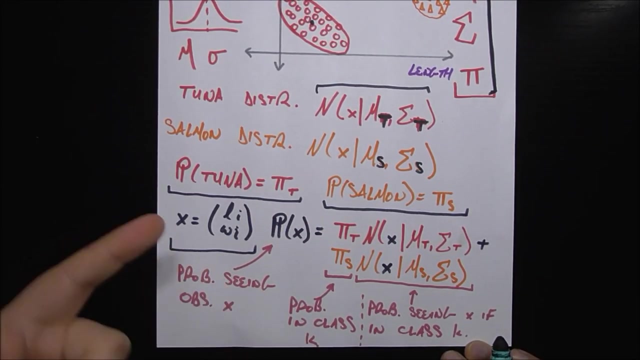 that means that if you give me basically all these points right here, all these tuna and all these salmon, I want to maximize the probability of seeing those examples, given some mu, sigma and pi. So that'll make a little more sense as we go through this example. So take one random. 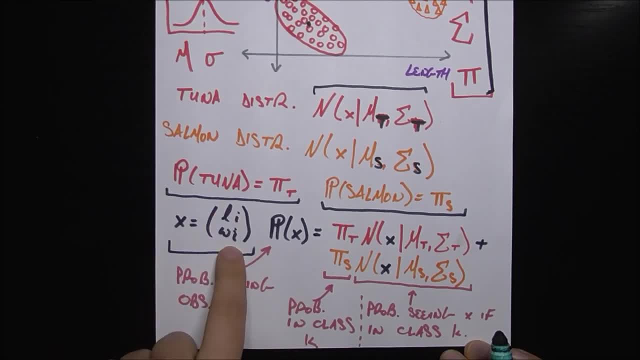 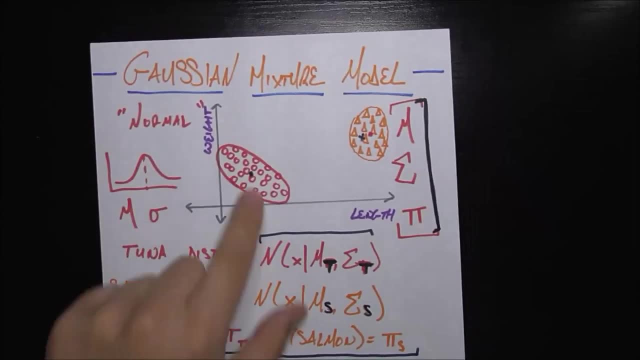 observation right. So if you have one observation x, with its length and its weight, what's the probability of seeing observation x? Well, there's two cases: Either that observation was generated from the Tuna distribution or the t, and it's the same observation, So we can do the same thing. So 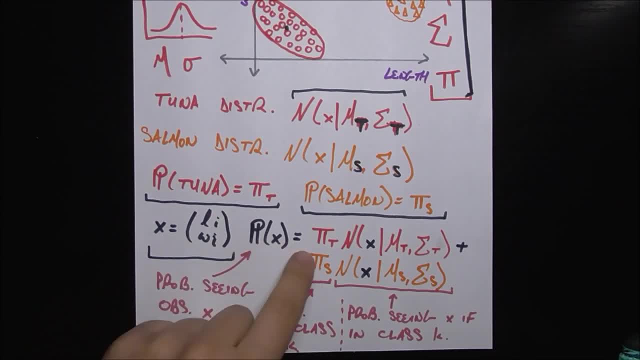 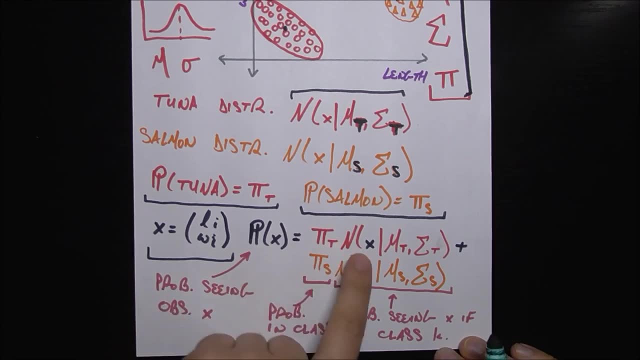 salmon distribution. So the probability of being generated from the tuna distribution is pi sub t. and if it was generated from the tuna distribution then the probability of seeing that example would be the normal distribution of x, or basically the normal distribution of the tuna generating x. So 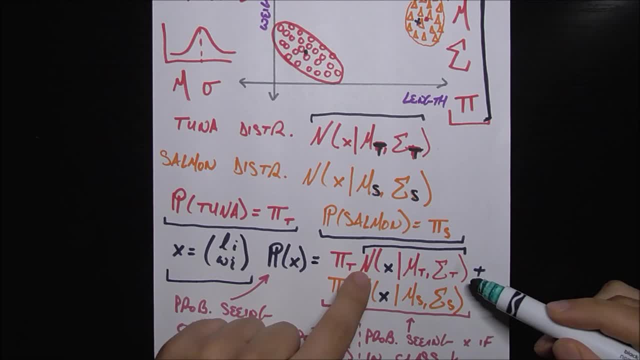 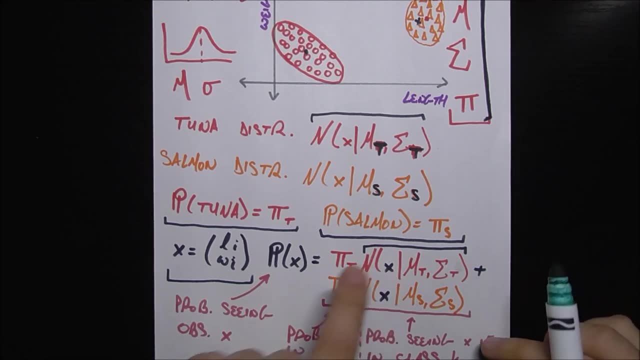 that's what this means right here. That piece right here means that, given that I'm from the tuna generating distribution, what's the probability that I get this value x? Okay, and I add that because I have a second case. I add that to the probability of something of this thing being a. 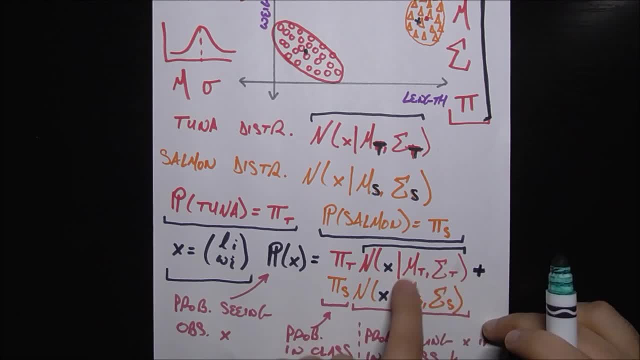 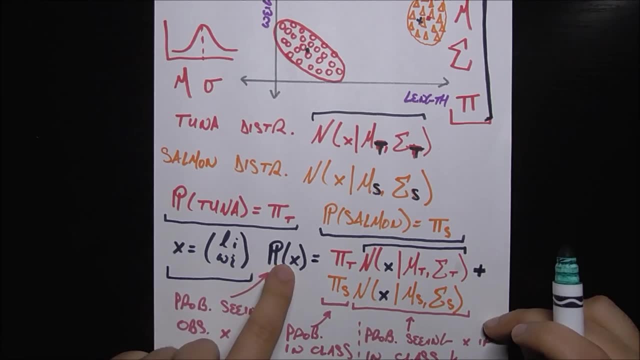 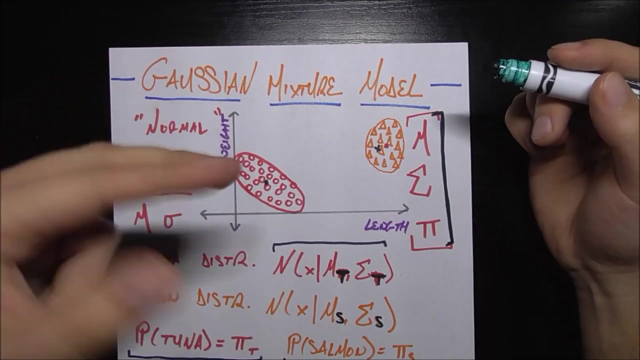 salmon times the probability that, given I'm in the salmon generating distribution, the salmon generating normal distribution, that it generates this value x. So that's the probability of seeing observation x and that is something I want to maximize because I truly did see observation x in the real world. I was given this observation and it truly exists. So I want to tweak my parameters. 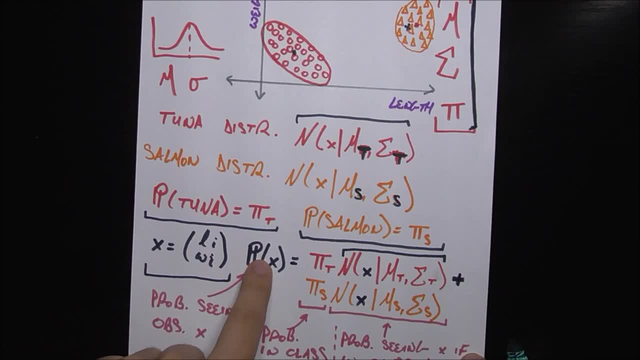 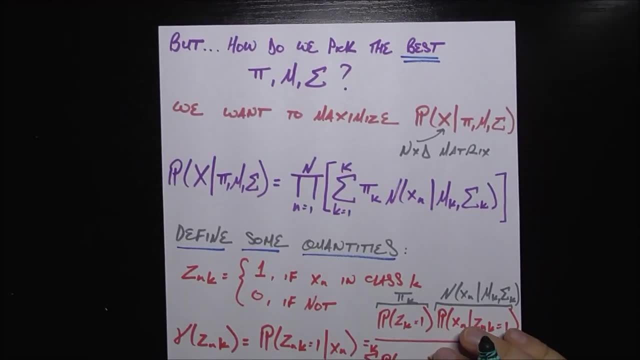 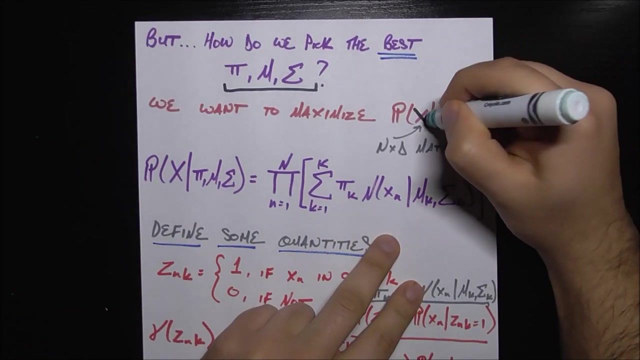 mu, sigma and pi such that they give me the highest value of actually seeing this thing that really exists. Okay, so let's switch over to this piece of paper and continue that conversation. So again, how do we pick the best pi, mu and sigma? That was a single observation, little x. here is a. 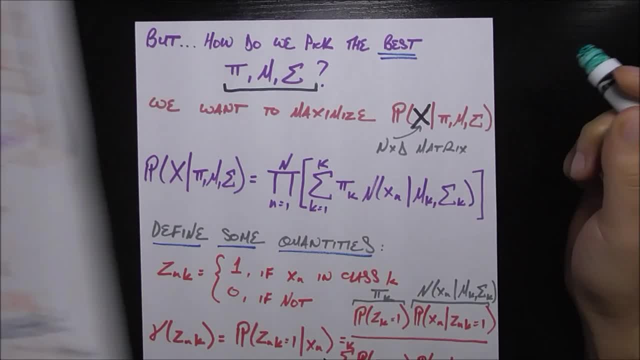 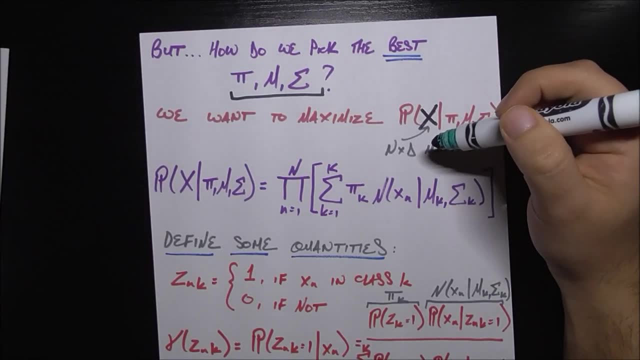 big x, which is an n by d matrix, n being the number of points, so that's all of these salmon and all of these tuna, and d being the number of dimensions, which is two. Remember, we have just a length and a weight for each fish. So, given that whole array of observations, given all of those fish, with all of 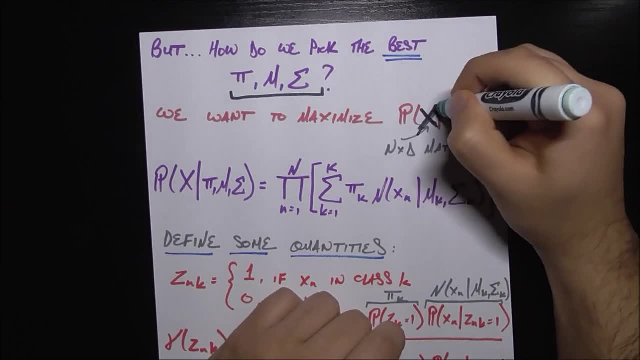 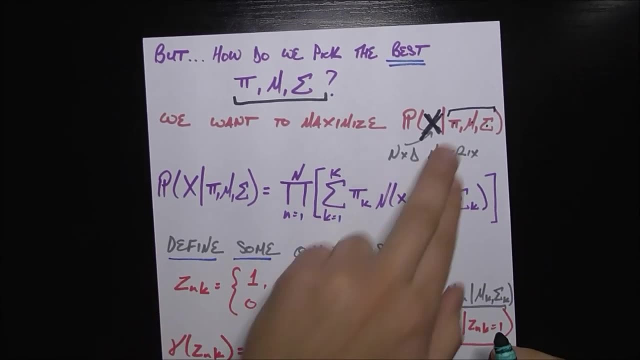 their lengths and all their weights. I want to maximize the probability of seeing all that data, given the parameters I have: pi, mu and sigma. So how do we have a more mathematical form for this? How do we expand this out? That's what's written on this line right here, and this is as mathy as 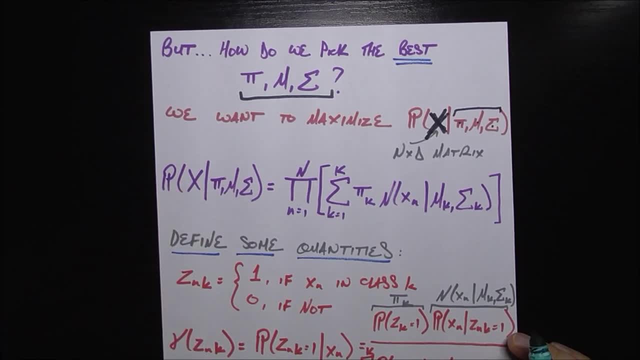 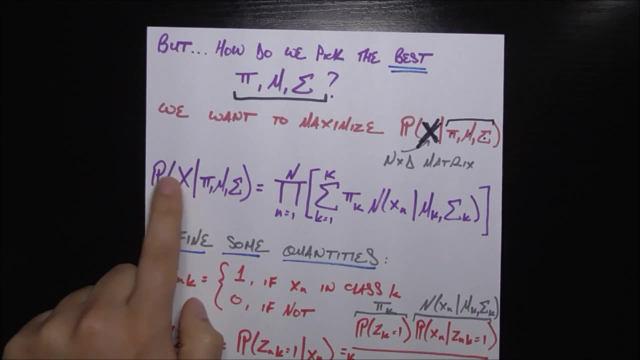 we're going to get. We'll see that if we truly want to maximize it, we're going to have to use some calculus. it's going to get pretty complicated, but we'll we won't go into that. So before we talk about that again, the probability of seeing this big x, all this data we have, 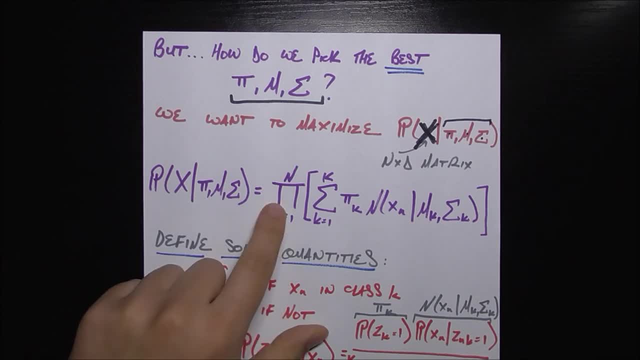 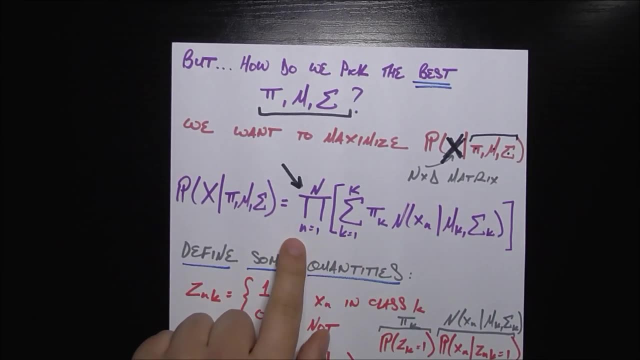 Given the pi, mu and sigma that we currently have is going to be so this outer pi. if you're not familiar with this notation, this is simply like a sigma, except you multiply everything inside instead of add. So here we're going, from n equals one to big n, which is all of the data points we 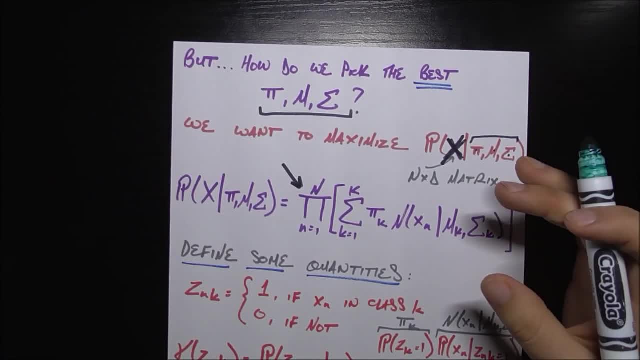 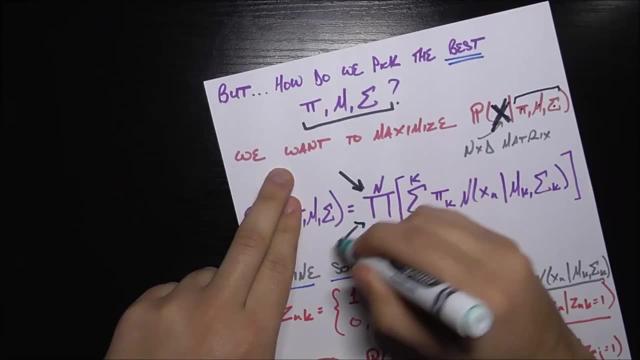 have. So we're assuming they're all generated independently. Okay, that's one of the assumptions of this model. So each one, the probability that we get for it, is going to be multiplied together. That's what this pi means. So I'll put: this is because of independence. 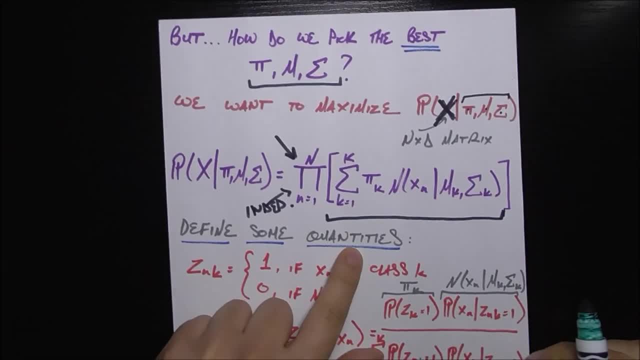 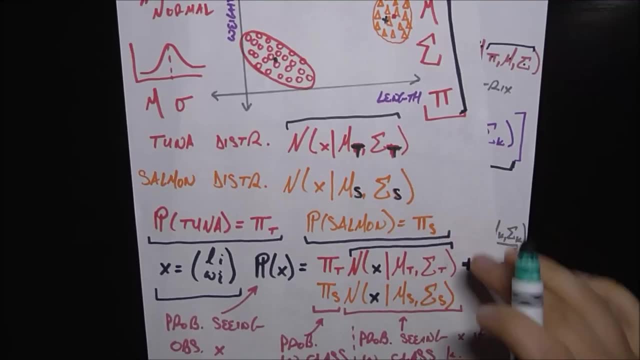 Now, for each of these two pieces, we're going to have to multiply them. So we're going to have to multiply each data point here. Now we're talking about any one specific data point in that set. We're basically just doing the calculation from the previous sheet of paper. So right here, remember. 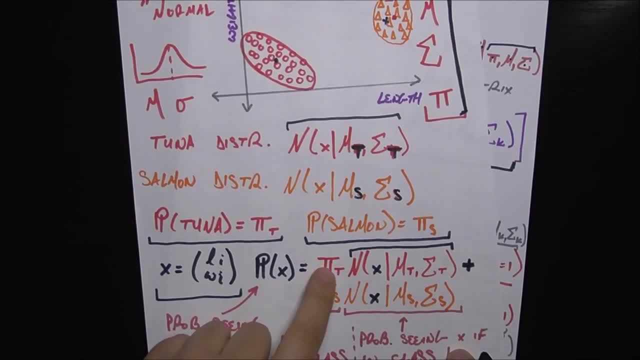 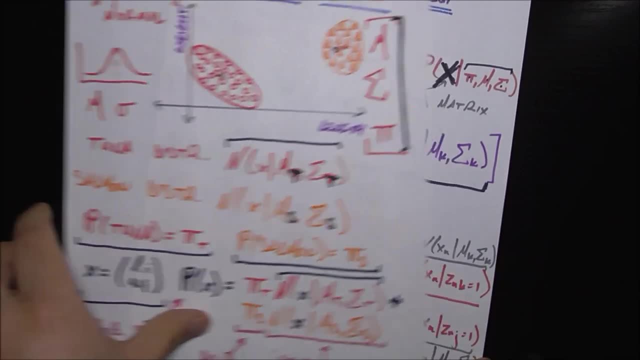 the probability of seeing any individual observation. x is simply just the sum of all the different classes. it can be, in times, the probability of seeing that observation, given that you're in this class, which is just the normal distribution right here. So that's what this is doing. This is. 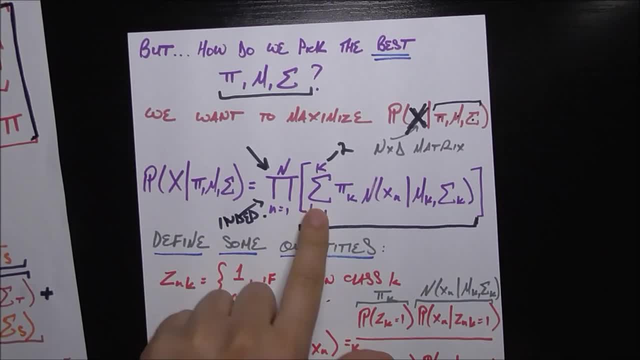 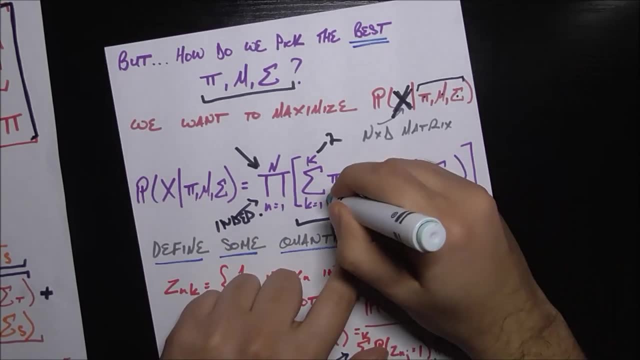 a more generalized form. Of course, for us k is just two, So I could have just written two terms. But this is in general for big K classes. It's the probability that this observation is in that class, which is pi sub k times. given that it's in that class, What's the probability of that specific? 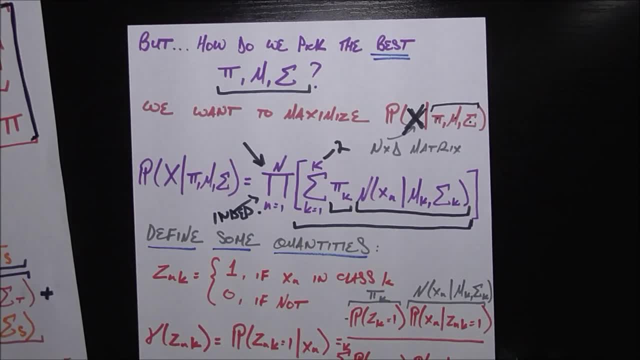 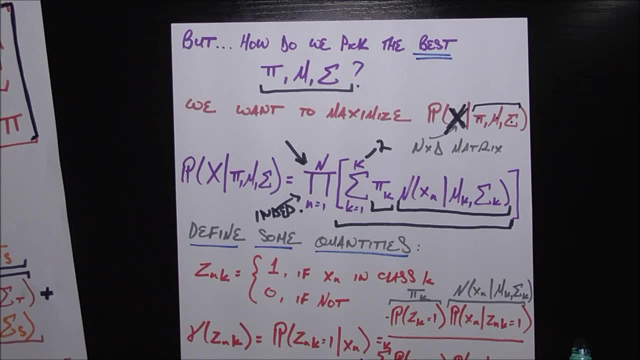 normal generating distribution, generating that point. So that's why we have this full form here. That's the probability of seeing the data we currently have, given this pi, mu and sigma. Okay, so before we go forward, what we're going to do is define some auxiliary quantities which will 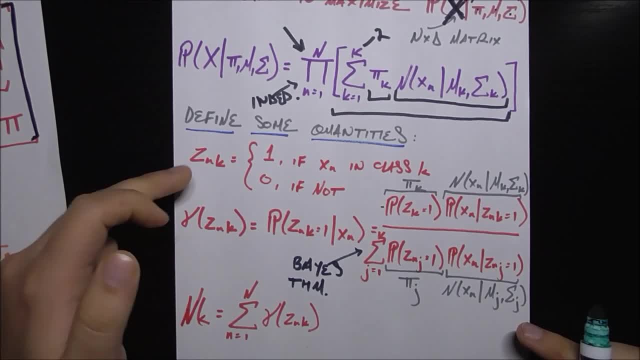 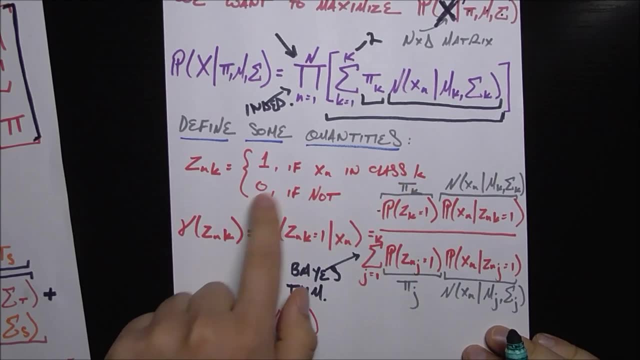 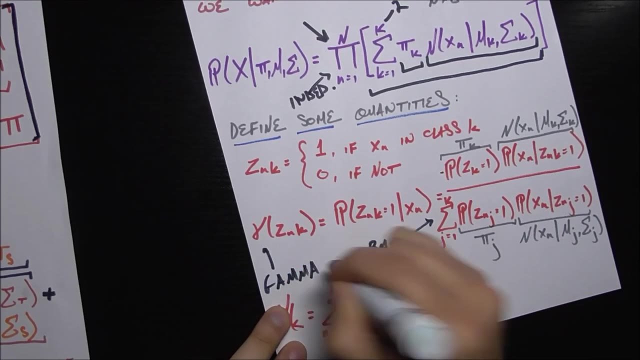 show up in our final solutions. Z sub n- k is really simple. It's an indicator variable, which is one if x sub n is in class k and zero if it's not. So just indicator. This Greek letter is gamma, if you're not familiar. So gamma of z sub n- k is simply just the probability that our observation. 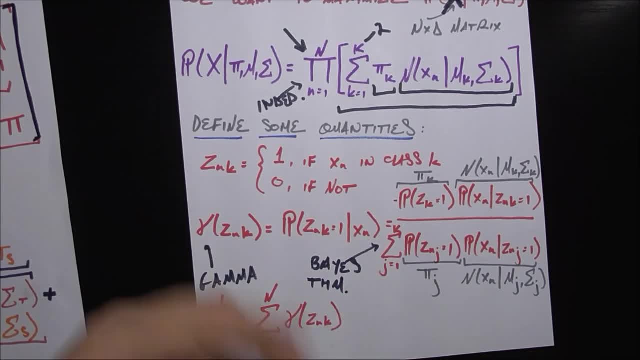 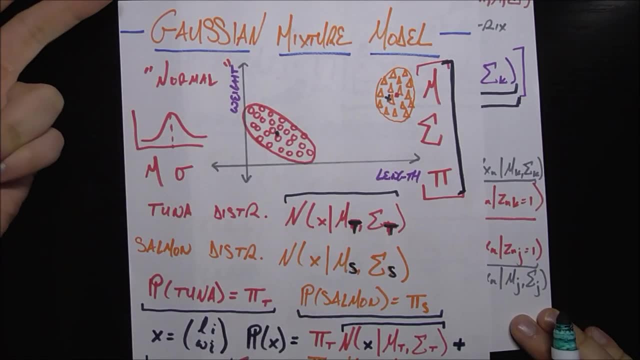 is in class k. Okay, given our observation. So basically, if someone gives you a new observation, this mystery point Right here with its given length and weight, and says: what's the probability that it's a salmon or what's the probability it's a tuna, That is basically what gamma z, sub n, k, where k is either. 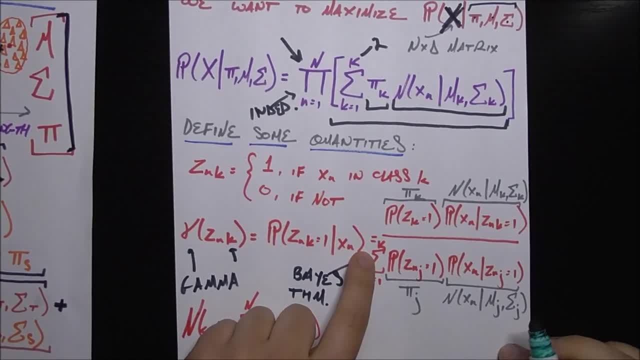 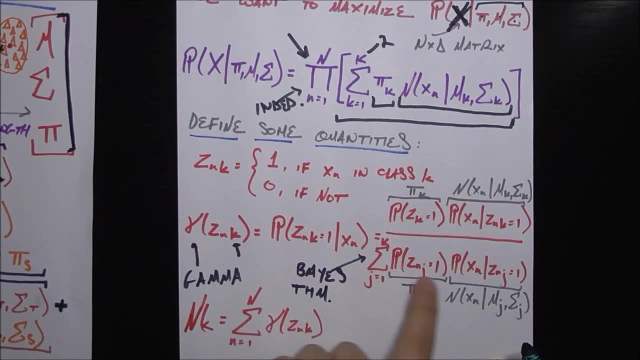 tuna or salmon. Okay, we can expand this out. This looks really scary, I agree, But you can go ahead and prove this for yourself using Bayes theorem. That's how we get all this stuff in red, But all this stuff in gray is just a different name we have for it. For example, probability that z k equals. 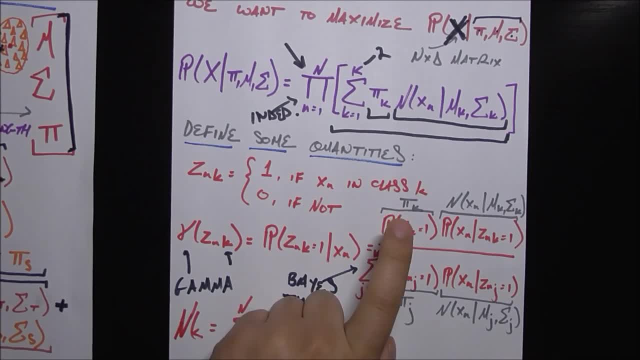 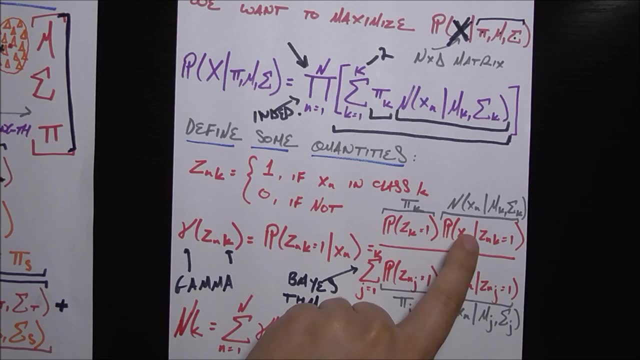 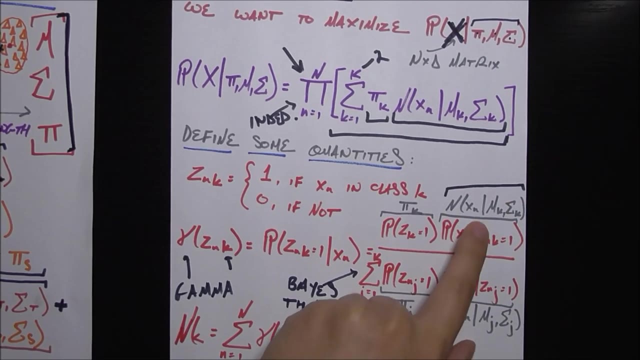 one is simply just pi k, Because it's the probability that any observation is in class k. That's just pi sub k. So we have a shorthand. And another thing here is probability that given something is in class k that we see that observation would just be the normal distribution for class k generating that observation. 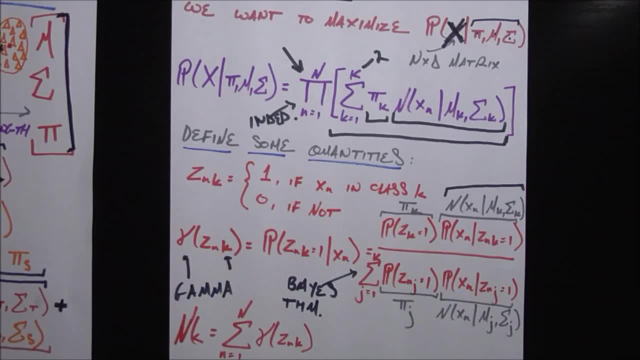 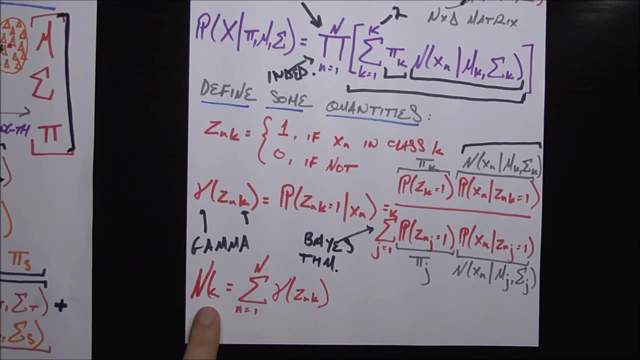 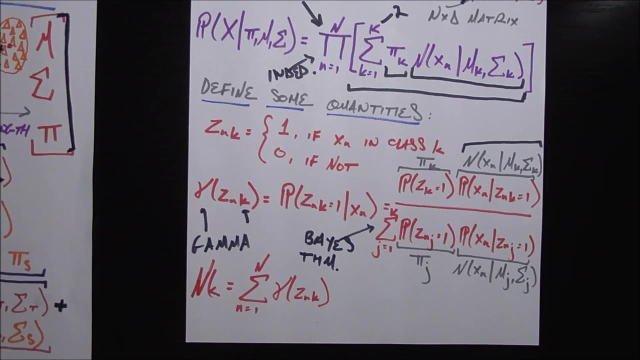 And similarly for these terms down here. So go ahead and verify that for yourself if you'd like. And this, going from this step to this step, is using Bayes theorem. The last thing is: n sub k is simply just the sum of Gamma z sub n k. going from n equals one to n. Okay, So these are some auxiliary quantities You're. 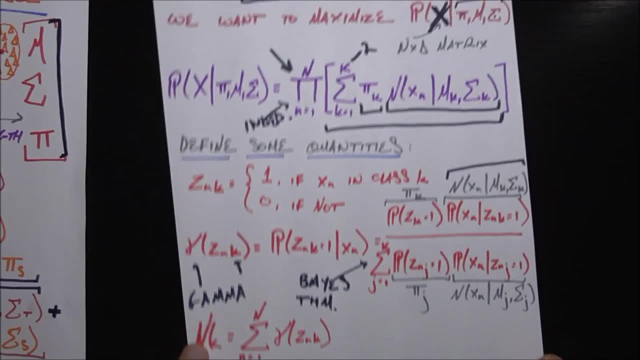 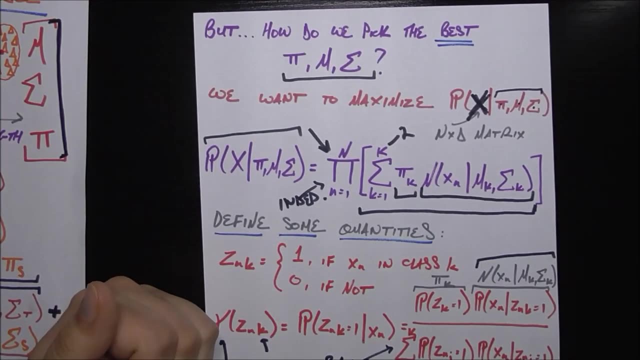 probably wondering what's the point of defining them. So the point of defining them is that, basically what we're doing here, we want to maximize this probability. Right, How do you maximize things in math? You take the derivative. So this is where it gets complicated. But basically, 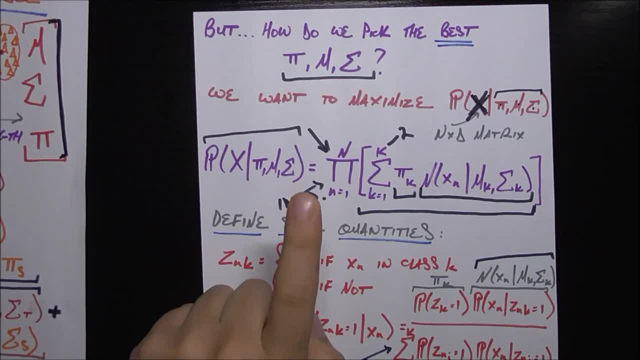 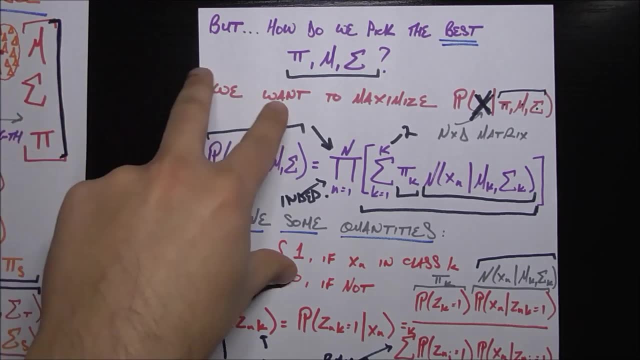 you can think of it as we're taking the derivative of this whole thing, basically with respect to pi sub k, with respect to mu sub k, in respect to Sigma sub k, separately and setting those equal to zero, And then we're solving for the optimal mu. 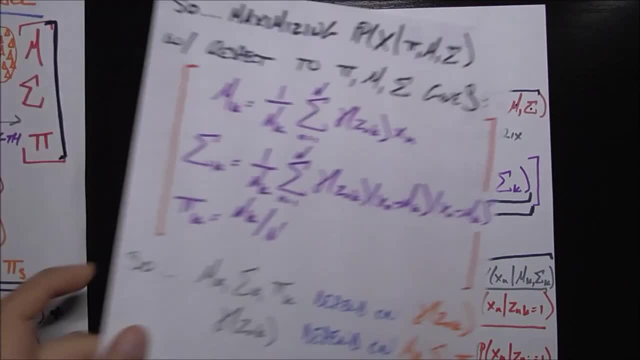 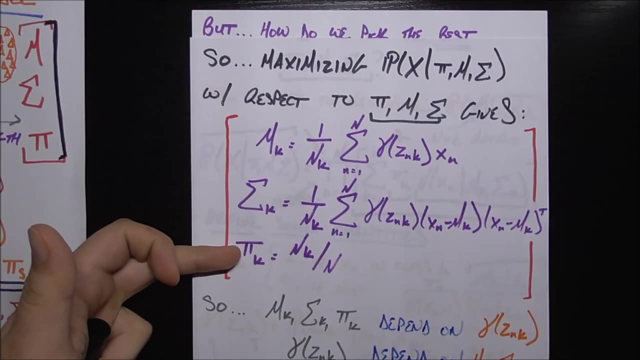 sub k, sigma sub k and pi sub k. And when we do that, this is what we get. So maximizing this guy with respect to all these parameters right here, gives us these three formulas for the optimal mu sub k, sigma sub k and pi sub k. And now you see why we had to define those quantities, because they show up. 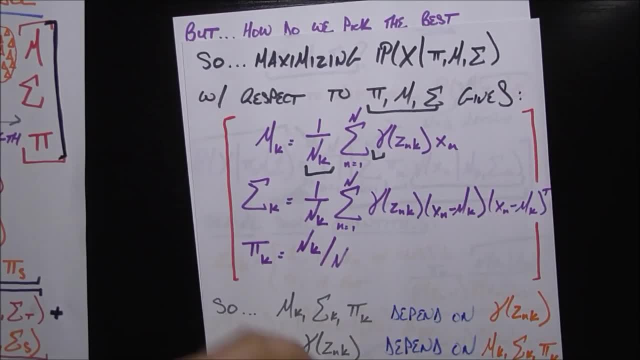 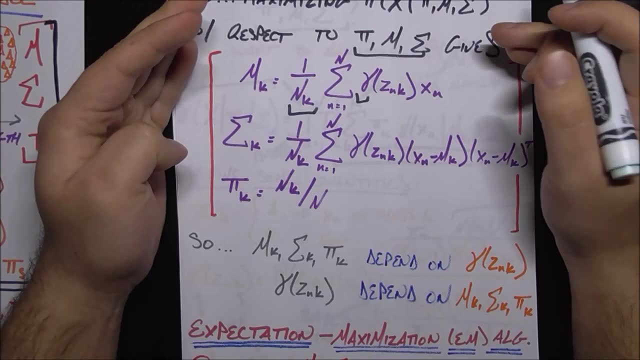 all the time. Here's n, sub k, Here's the gammas, for example, So they're showing up all the time in here. That's why we needed to define OK. So basically, this is all very complicated and you can go into it more if you want. There's many. 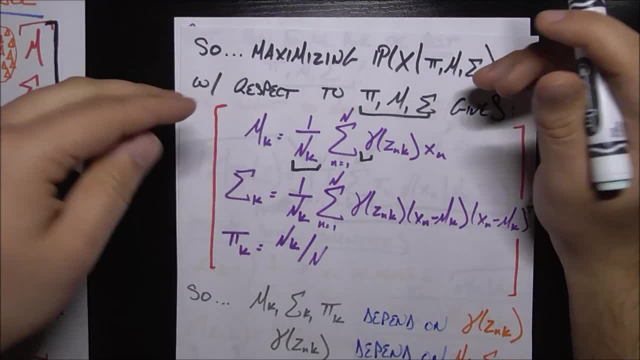 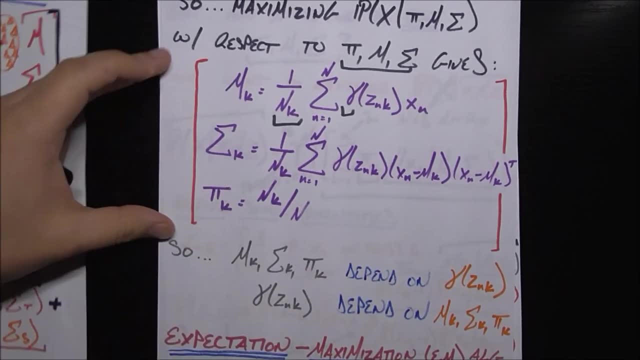 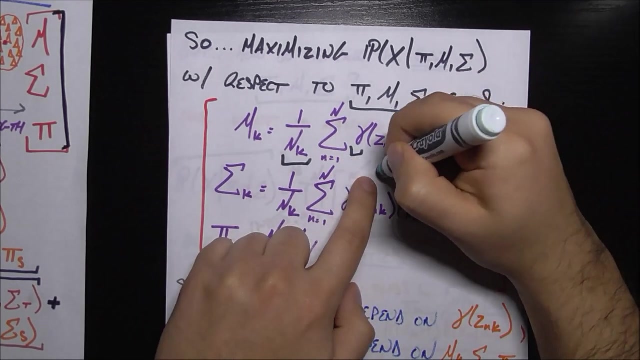 resources out there for all the math. You can go through it, verify it for yourself, But at a high level. what we need to notice is that the formulas for mu sub k, sigma sub k and pi sub k, that is, these three up here- only depend on this gamma Right, Because here we see that we would need to know. 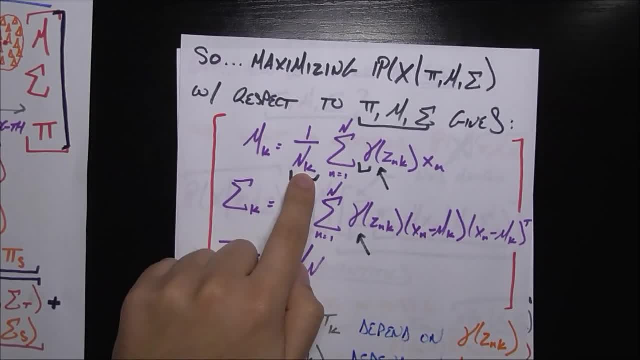 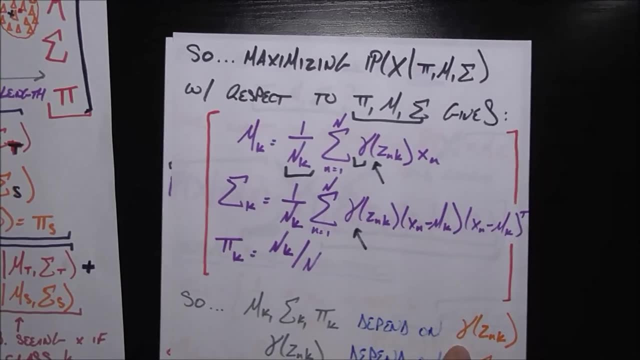 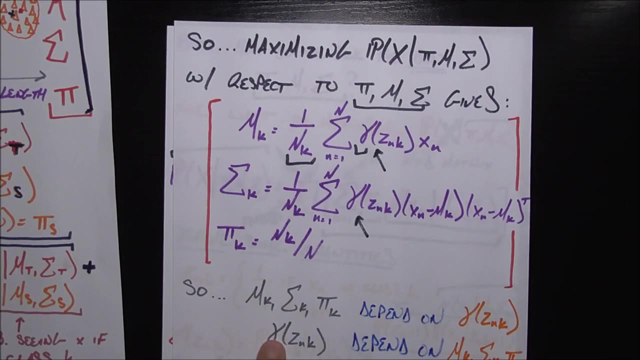 this gamma here. We would need to know this gamma here, This n sub k. you say, oh, that does that depend on gamma? Well, if we look at this, this n sub k indeed, just depends on gamma. So if we know the gammas, we already know mu sub k, sigma sub k and pi sub k, Also this gamma. Let's look at the. 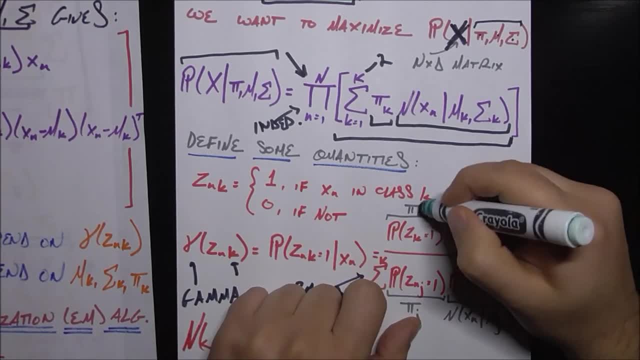 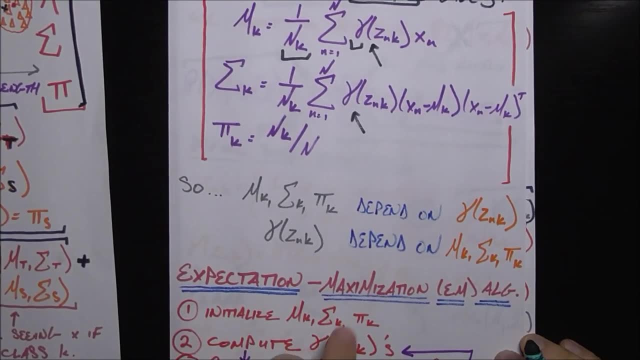 formula for that gamma, which is right here That only depends on the pi sub k, is the mu, mu sub k's and sigma sub k's. So they kind of depend on each other. That is, if we have the gammas we can calculate these three guys, And if we have these three guys we can calculate the. 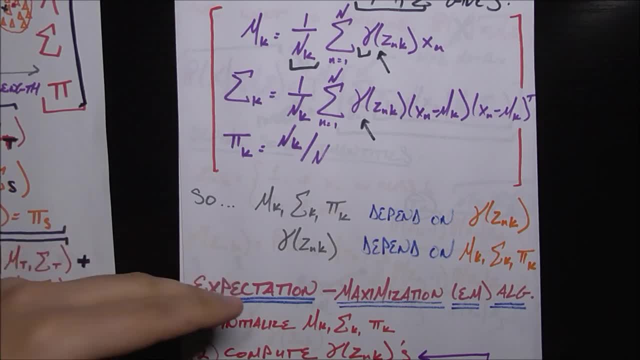 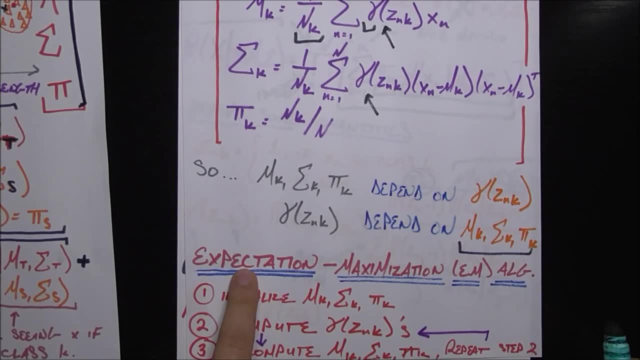 gammas. So it seems like a circular dependency. But another way to think about it is just a formulation for an algorithm to find the best values for our parameters, And the algorithm is called the expectation maximization or EM algorithm, And it's just three simple steps. 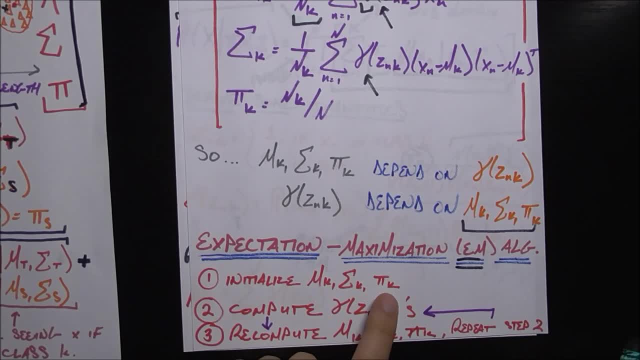 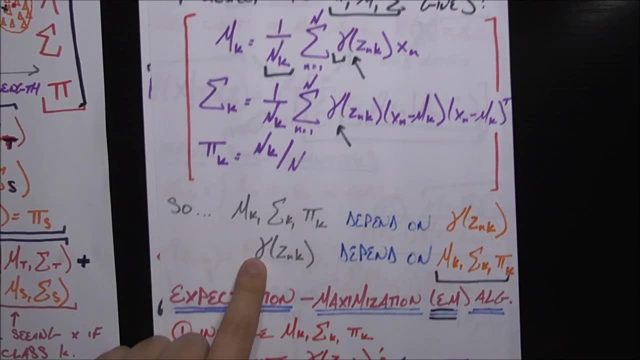 The first one is we initialize mu sub k, sigma sub k and pi sub k to some values that make sense, whatever initial values we want. Next, remember that if we have these, we can successfully calculate our gammas. So we go ahead and calculate our gammas in step two. 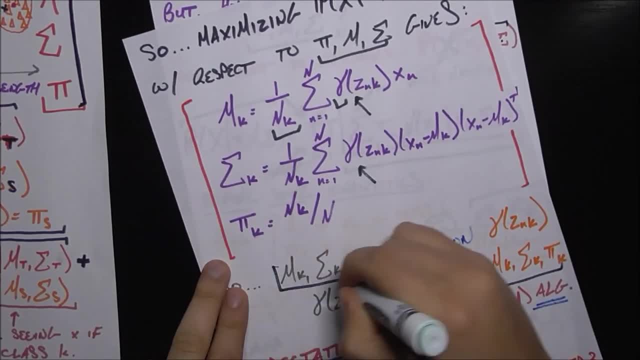 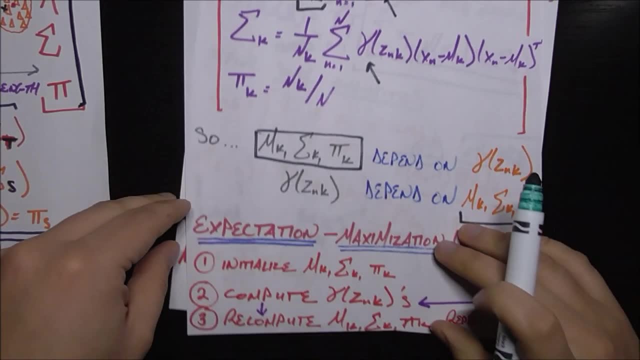 Now that we have our gammas- remember, we can recalculate these three parameters here Because we had some initial values for them, but with our gammas those values are going to change a little bit or a lot. So in step three we recompute mu sub k, sigma sub k and pi sub k. Now that we have 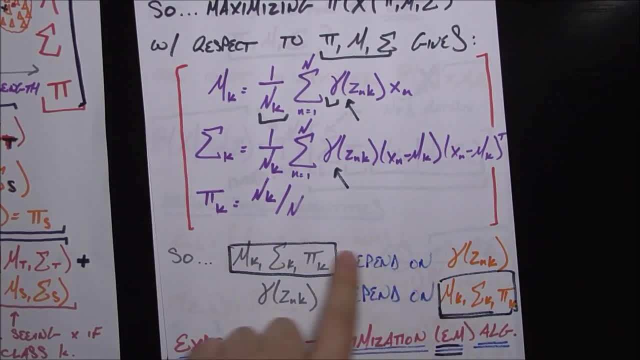 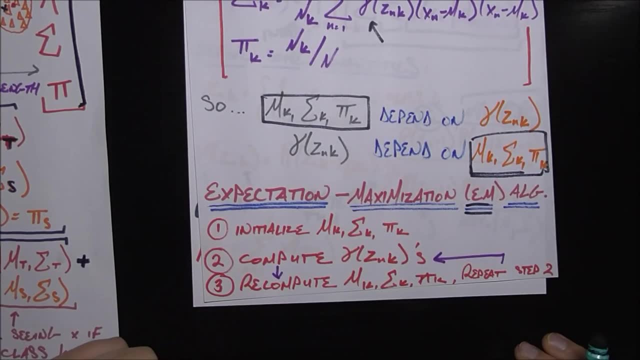 new values for these guys. we can basically just repeat: right, We can recalculate our gammas, And then, now that we have new gammas, we can recalculate these guys. So we can go again and again, and again and again, right, And you're basically asking: when do I stop? Well, there's different ways to do that. 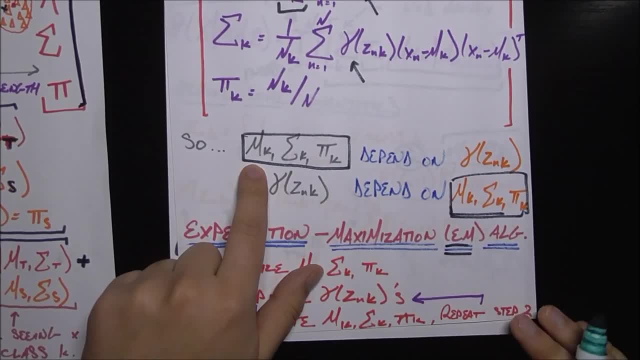 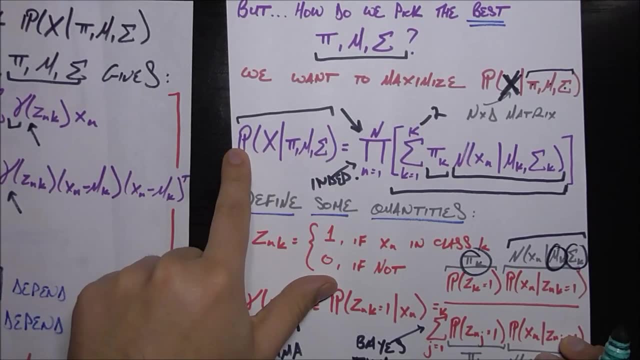 There's different stopping criteria you can set. One would be these parameters converge to something. You could also say that the function you're trying to maximize, for example this function right here- that converges to some maximum. Or you can set up some other stopping. 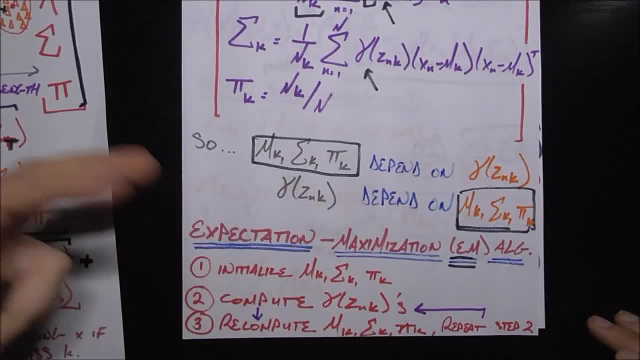 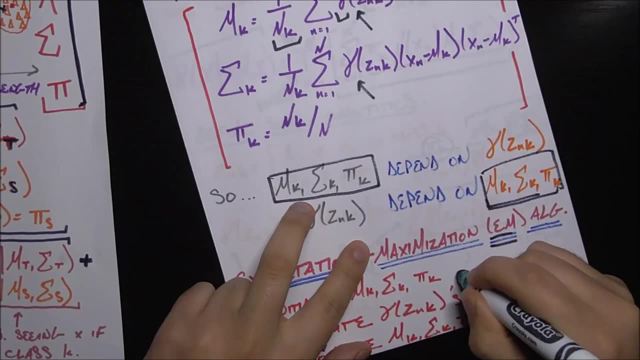 criteria altogether, Just do a thousand or ten thousand iterations, So anything that makes sense to you. Okay, But that's what the EM algorithm is, And I should say that. so step two is the E step, the expectation step, And then step three is the maximization step, Because in that step 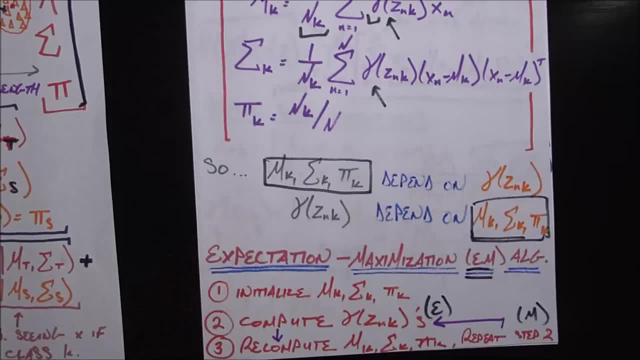 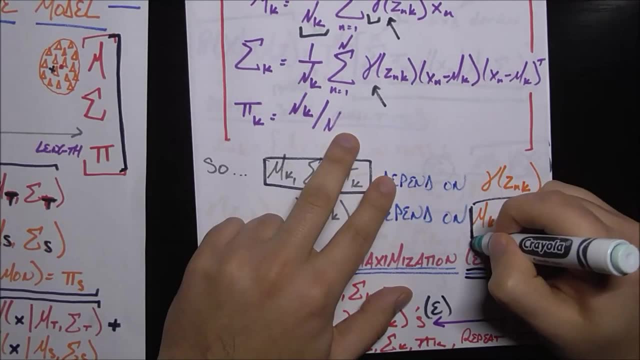 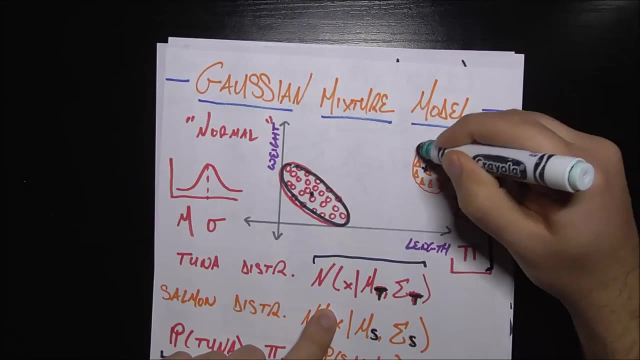 we're picking the parameters which maximize our function. Okay, So that is basically how the Gaussian mixture model works. At the end of that, we have our best values for mu, sigma and pi, which hopefully match up to these visual distributions we see in our data set. Okay, And another question. 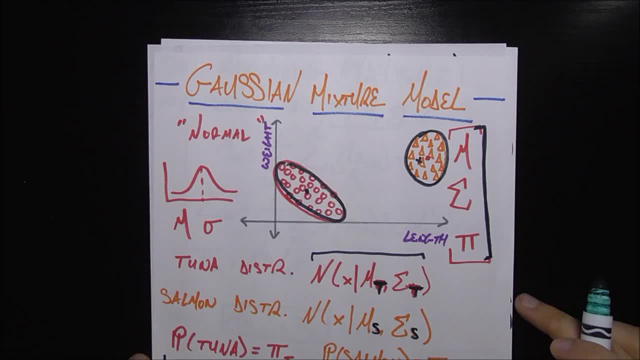 you're probably wondering is: why is the Gaussian mixture model useful? It was so much work, It was so much math. It's probably computationally pretty expensive. Well, something we saw in k-means is that k-means is problematic when the clusters are of very different sizes. Just for example, let's